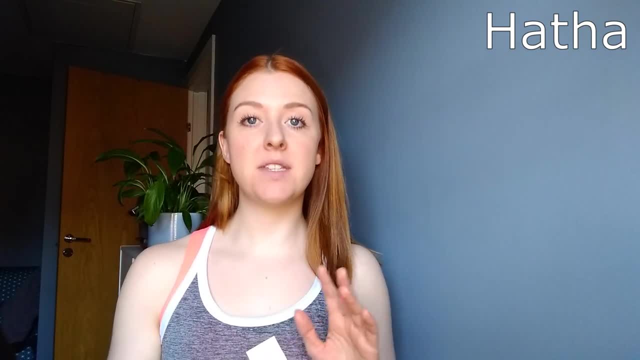 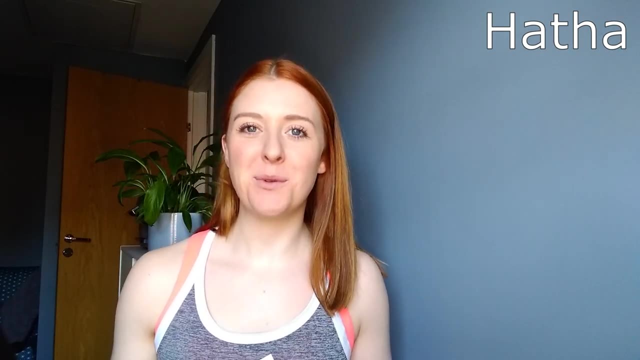 three to five breaths While you're in that pose. it gives the teacher an opportunity to break down exactly what all of your different body parts should be doing. For example, if you're in a warrior one pose, you would. the teacher will be telling you to have a bend in the front knee. 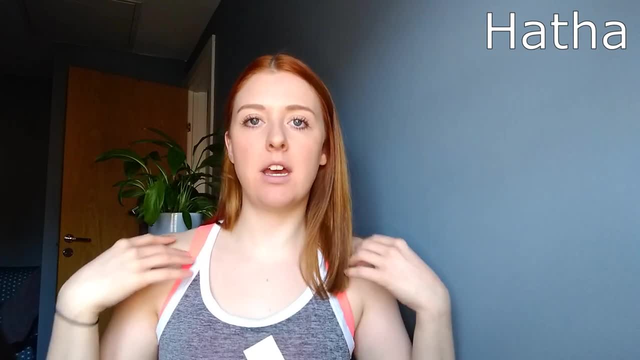 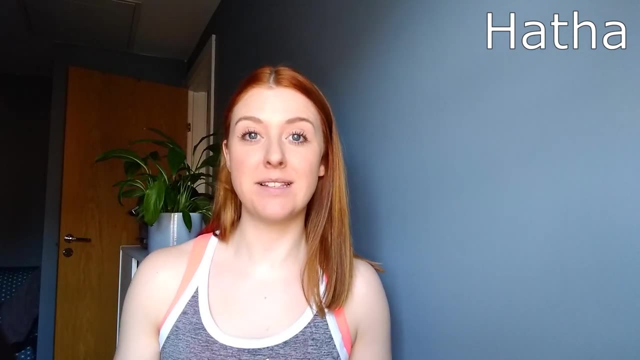 to check how, the placement of your back foot, to have the arms reaching up, to be aware of the shoulders, the core, and they can talk you through in detail, which is why hatha yoga is really good for beginners, because you get the chance to really understand what you're supposed to be doing in. 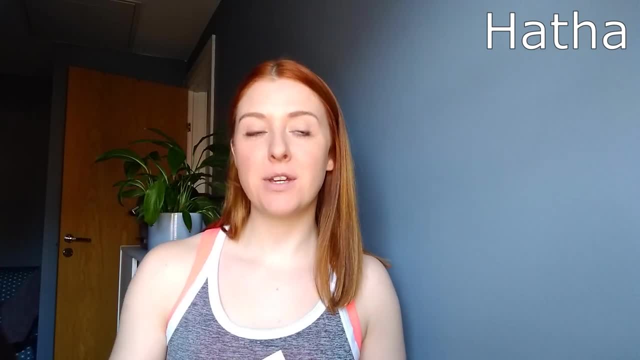 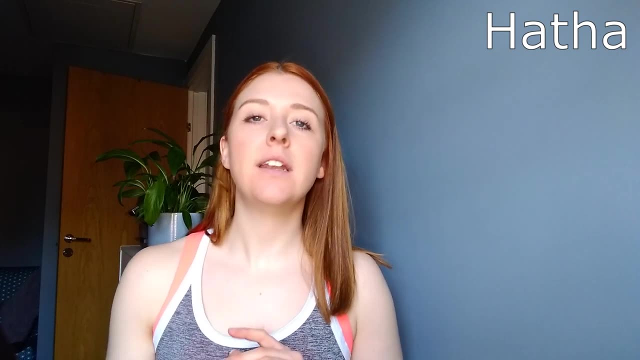 each pose before you move on to the next one. And then, with hatha yoga, you would do that pose on both sides and then you'd move on to the next one, and then the next one, and the next one. So you're unlikely to come back to the same pose twice within a class. You might do, but it's unlikely. 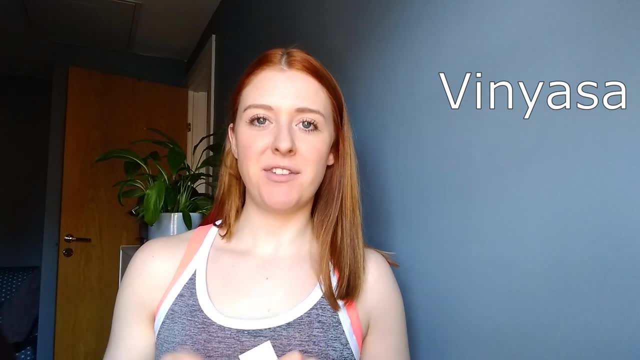 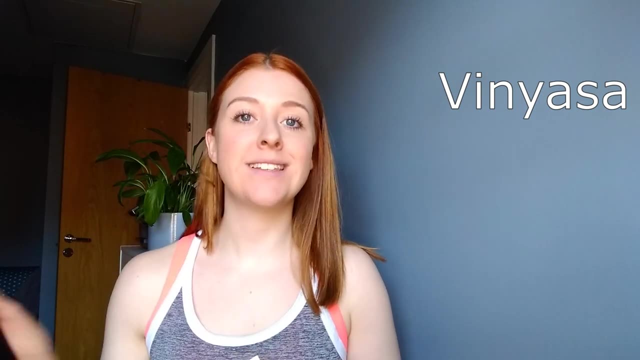 That takes us then on to vinyasa yoga. So second type of yoga, vinyasa. this is sometimes called flow yoga as well, and the reason for that is because it's a type of yoga that you can do is it's more of a flowing sequence. So, whereas with hatha yoga, you're likely to do a pose once, 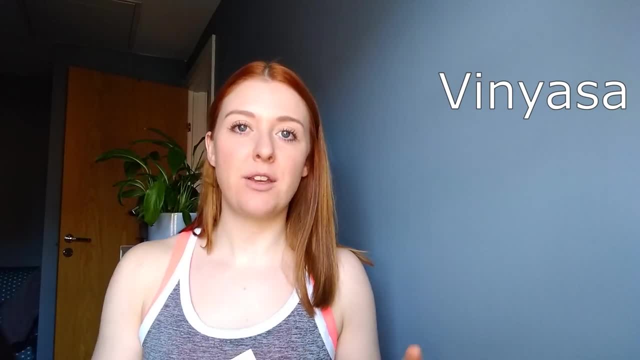 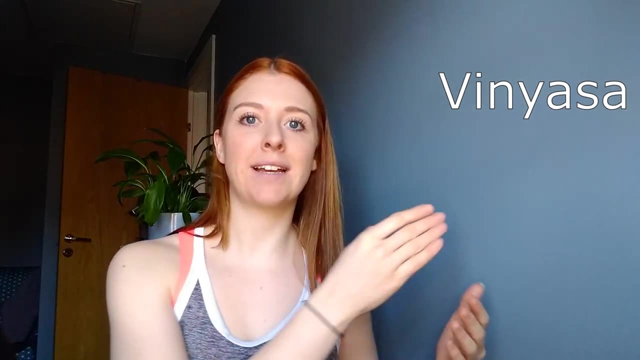 move on to the next one, the next one, the next one. With vinyasa yoga you would move through a little sequence, So you might do say, pose one, two, three, four, and then you'd come back and do those again, maybe adding on something a little bit different or adding in a few extra poses. 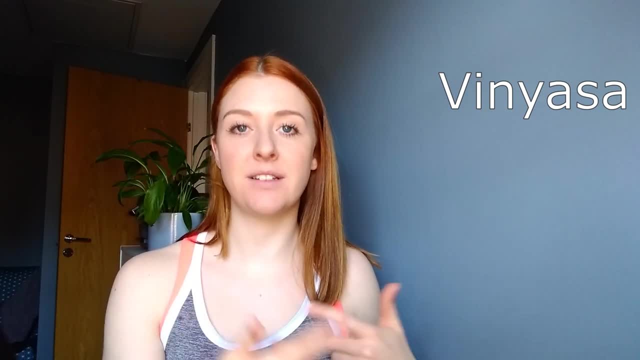 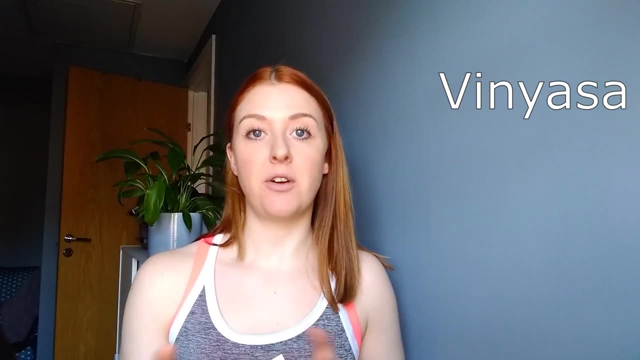 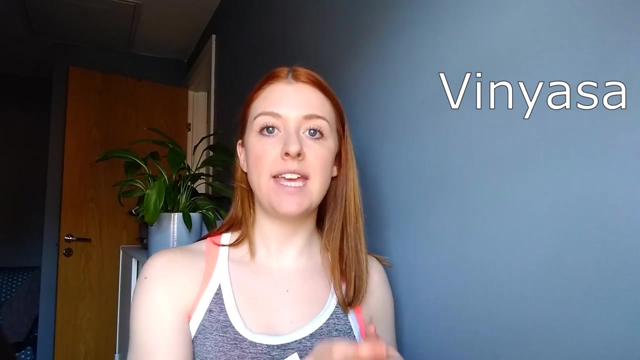 but you might repeat kind of a loop of poses, a little sequence as you go along, And with vinyasa style you don't spend as long in each pose. So depending on the teacher and the pace of the class, you might even just take a breath in moving into one pose and a breath out moving into the. 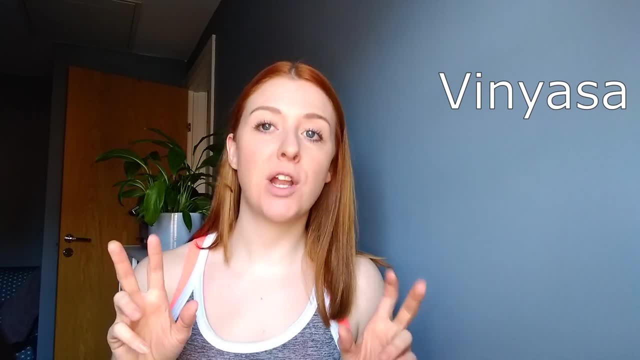 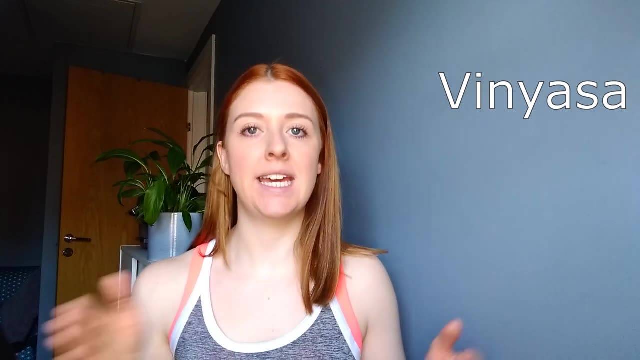 next, So it can be a really quick movement. There's also kind of slow flow yoga classes where it's slowed down a little bit more, So you would then spend a bit longer in each pose, but the same idea of kind of flowing through the different poses And, because of that, more fluid. 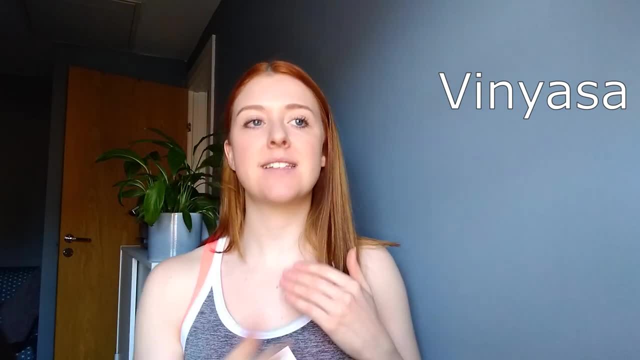 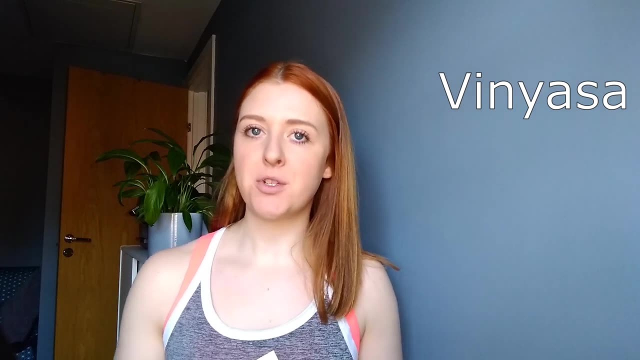 on the transitions as well, So moving from one pose to the next in a nice flowing, fluid kind of way. While vinyasa yoga is a lovely style to practice, it's maybe not the best option if you are a complete beginner, because the teacher doesn't really have time to explain in detail. 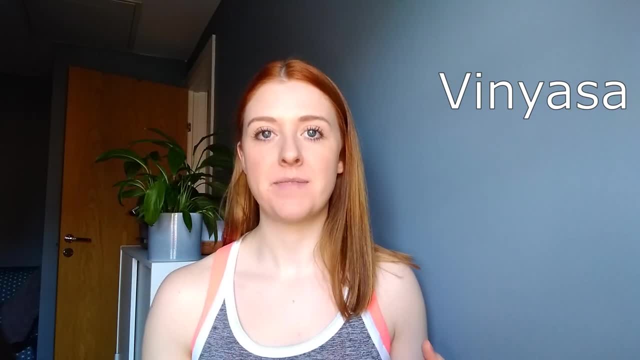 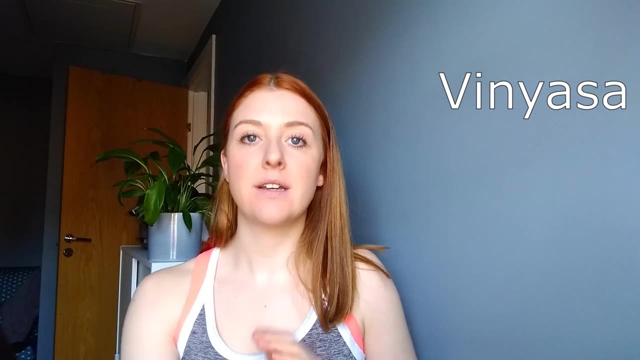 how to have correct alignment in each pose. So, whereas with hatha yoga you slow it down a little bit more and go a bit more into depth with the poses, with vinyasa you're moving through them fairly quickly, So you have to have a bit of an understanding of how to do it. So if you're 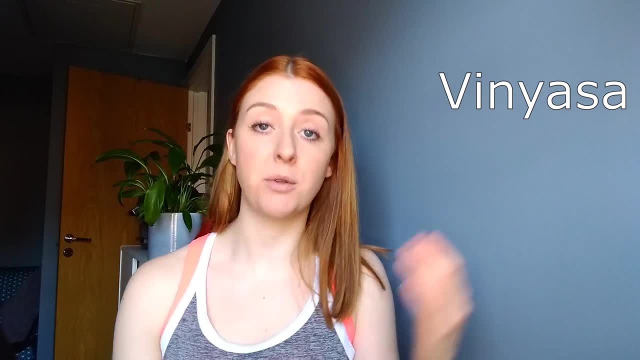 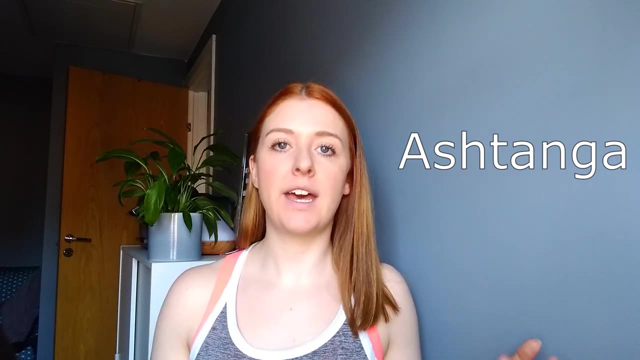 a complete beginner, you'll have to have a bit of an understanding of each of the poses before you would be comfortable going through that sequence, Then moving on to ashtanga yoga. So this is similar to vinyasa yoga in the sense that you move through in a kind of fluid, flowing kind of way, But the 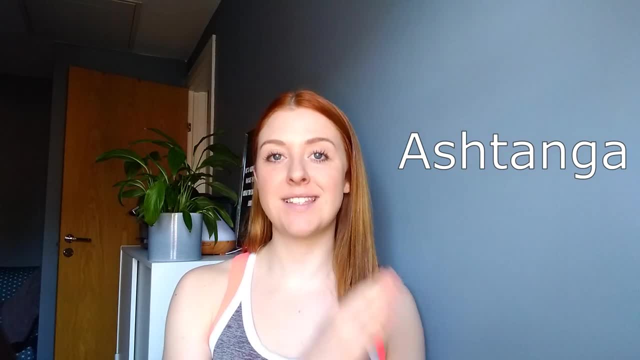 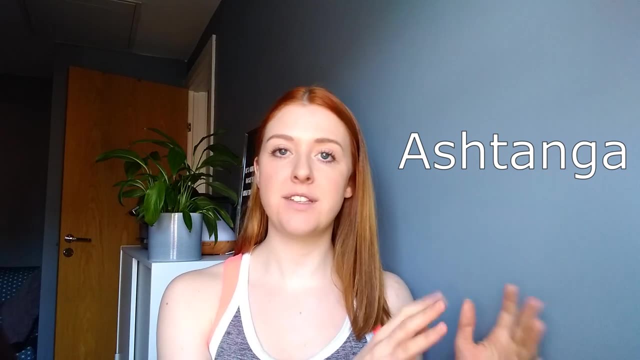 difference here is that with ashtanga yoga, you practice the set series or sequences that are always practiced in ashtanga. So with vinyasa yoga, the teacher has complete freedom to make up different sequences every week. You'll practice the set series or sequences that are always. 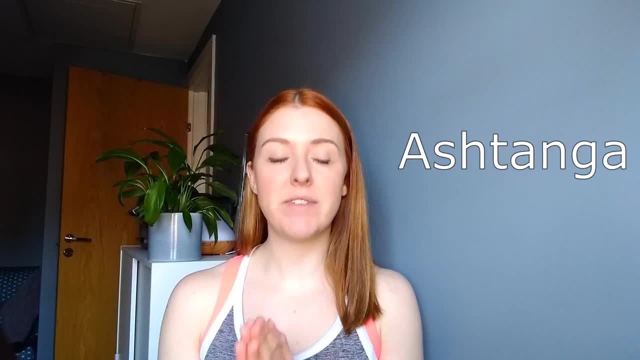 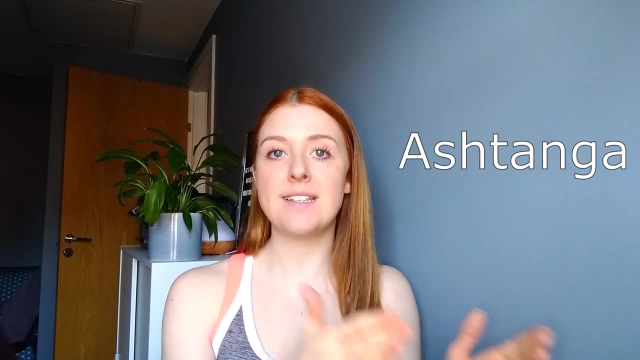 practiced, You'll practice lots of different things, Whereas with ashtanga yoga, every class you go to you're going to practice the same series. Now of course you have sort of a more beginner series and then gradually you can progress on to these more advanced series, and they do get really. 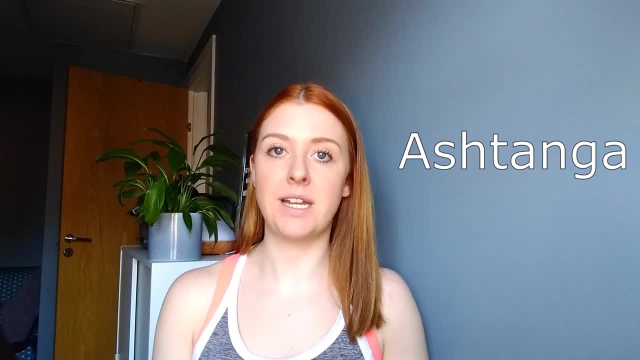 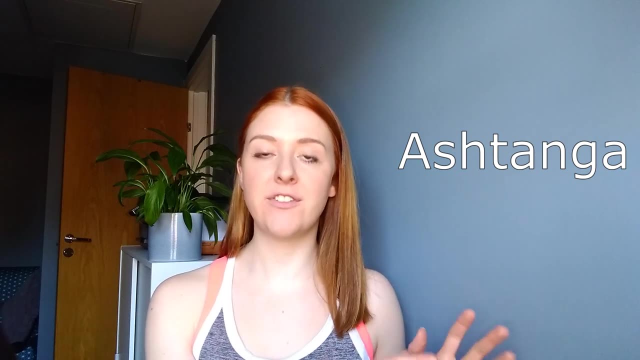 advanced, But the beginner series, the kind of primary series as they call it, is appropriate for beginners. It's challenging, though. I would recommend trying out some hatha yoga first, but then, once you're a little bit more familiar with how to do it, you'll be able to do it. So if you're 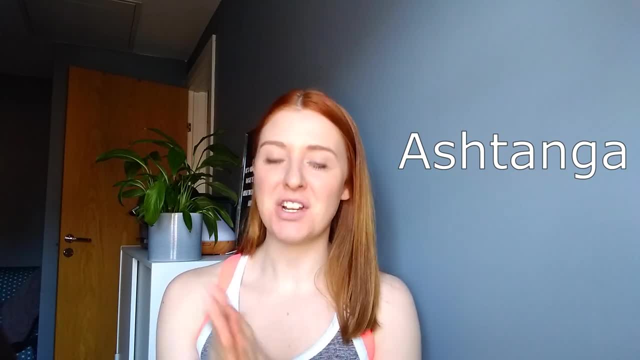 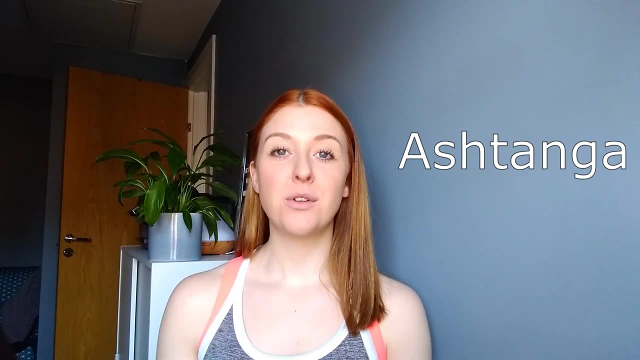 learning how to move your body and to breathe in the yogic way. ashtanga is a nice option if you're someone who likes a bit more rigidity and structure in your practice. So once you get the hang of this kind of sequence, this series, that is set and always stays the same- the nice thing about 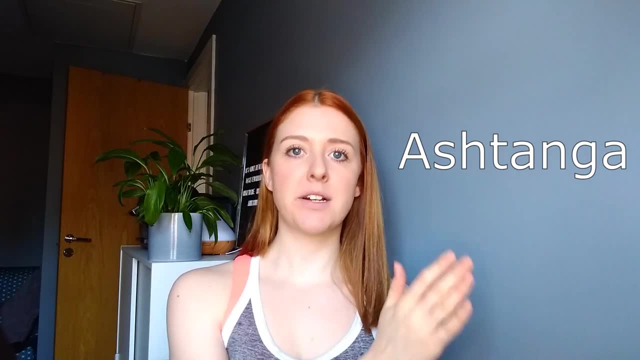 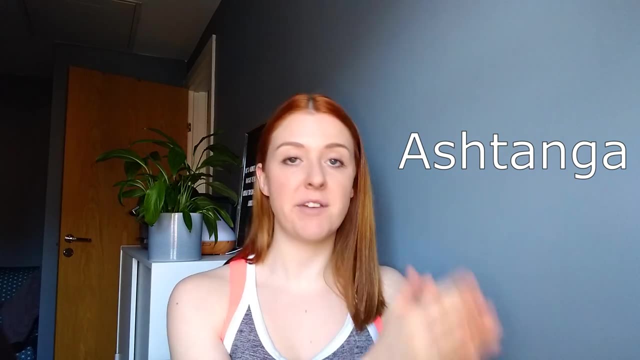 ashtanga yoga is, you can see a kind of marked progress from when you start to when you've been practicing for a little while. Because you're practicing the same poses, you probably notice that from the first time you try it to the 10th time you try it, you're going to notice that you're 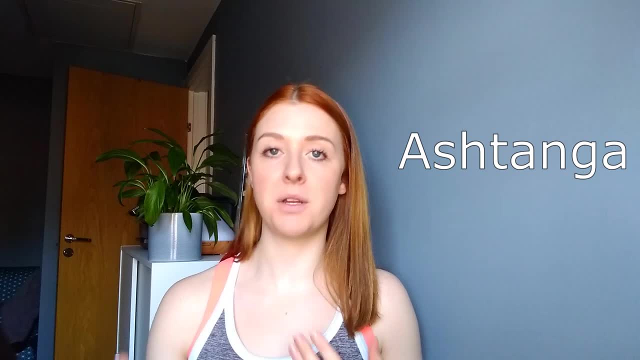 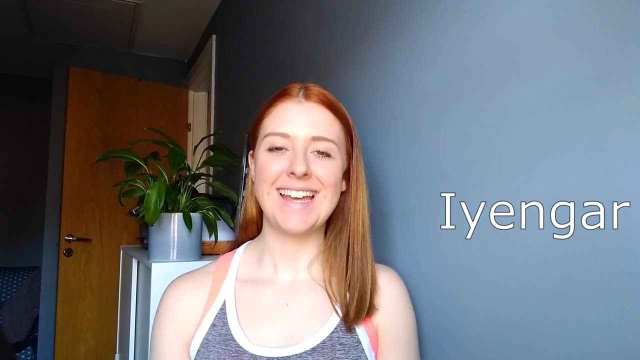 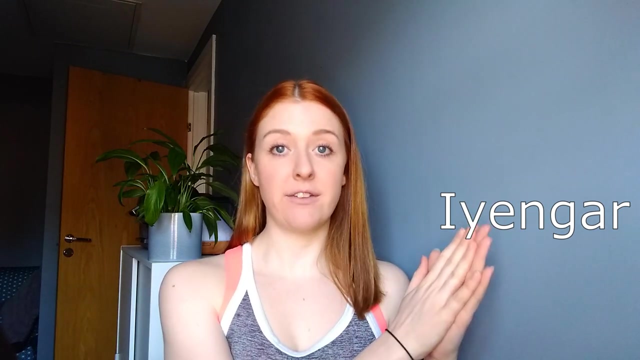 doing it the 10th time you try that series, There will be a huge difference and your body will be so much more strong, flexible, mobile and everything else. Next up is ayengar yoga, named after the man who founded this style of yoga. Ayengar yoga is closer to hatha yoga, I would say so. the first one. 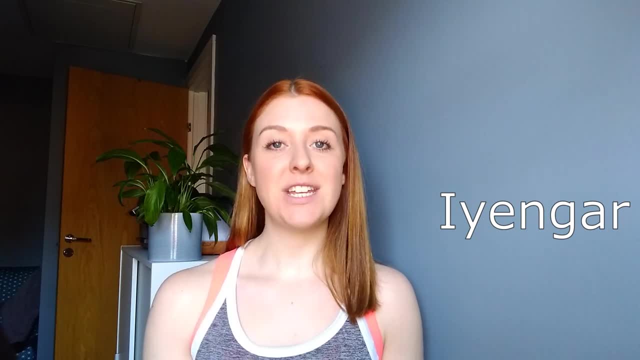 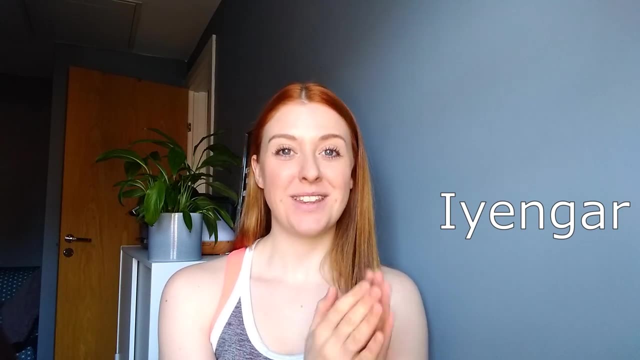 that we talked about, in that you're going to hold the poses for longer and the teacher is going to go into a lot of depth to make sure that you are holding the pose correctly. With ayengar yoga, they are more detailed than they would in a hatha yoga class, And with ayengar you're going to use more. 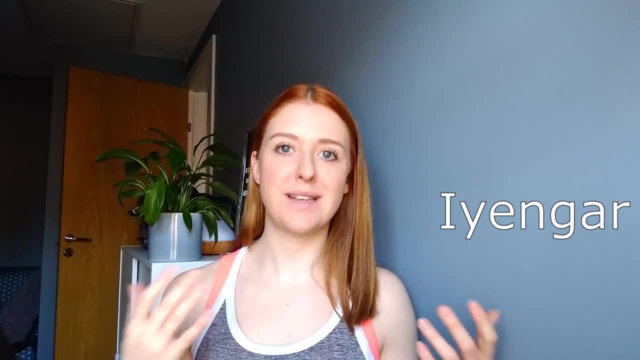 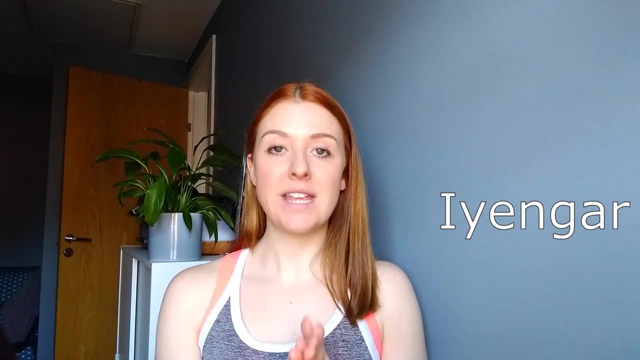 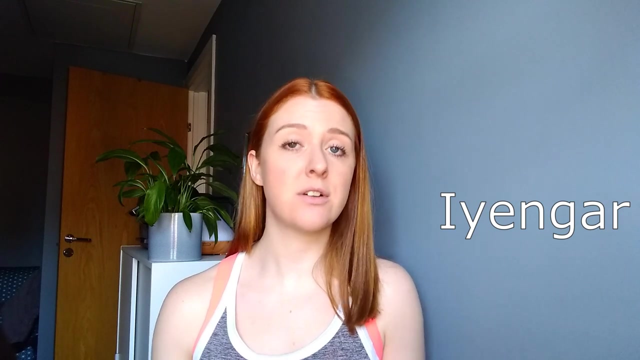 props, so things like yoga blocks, straps, bolsters, things like that to access the poses in the best way for you. So in that way, ayengar can be a really good practice for beginners or for anyone with injuries, I would say, Because, as long as you have a good practiced ayengar yoga teacher, 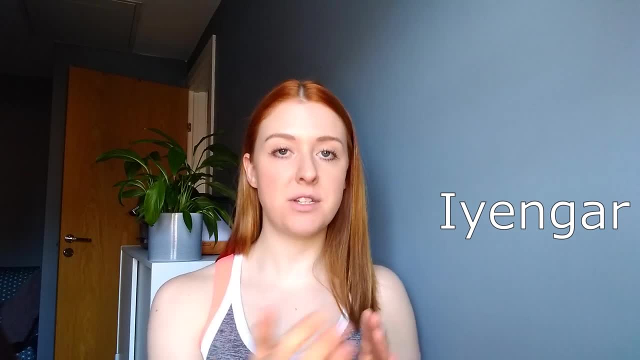 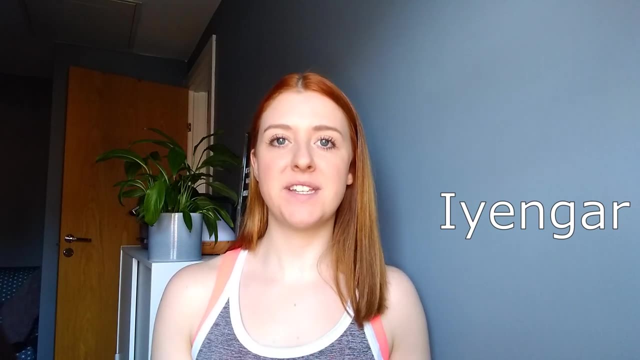 they should be going into enough depth that they will come around to each of you and make sure that you are into the pose in the best way that you can be for your body. The kind of emphasis in ayengar yoga or the thing that sets it apart from the other styles. 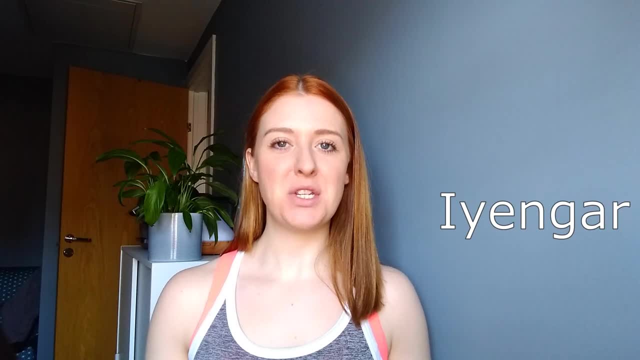 is the precision. So with an ayengar yoga teacher, you're not going to get away with any kind of sloppiness or laziness or bad habits. they're going to really be quite strict on making sure that if your arm is reaching up, it's straight and you're actively reaching up, you're not. 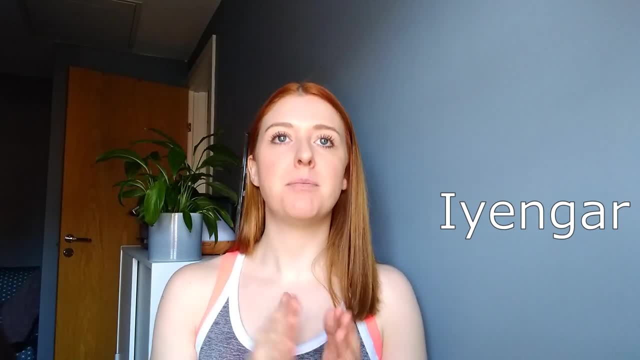 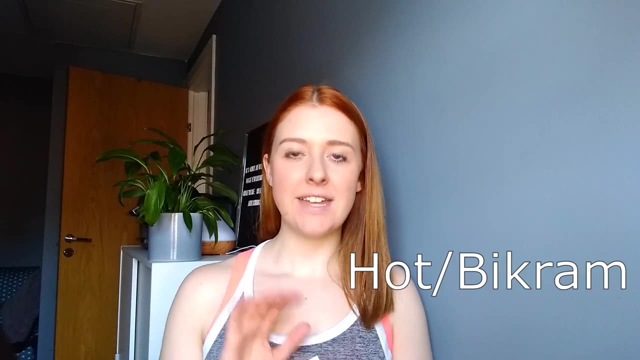 letting everything go a bit floppy, So it's a bit more strict, but it's a slow, strong practice and you will definitely build a lot of strength very quickly. practicing ayengar yoga, Then five out of six on this list is well. it's two styles really, but I'm going to categorize. 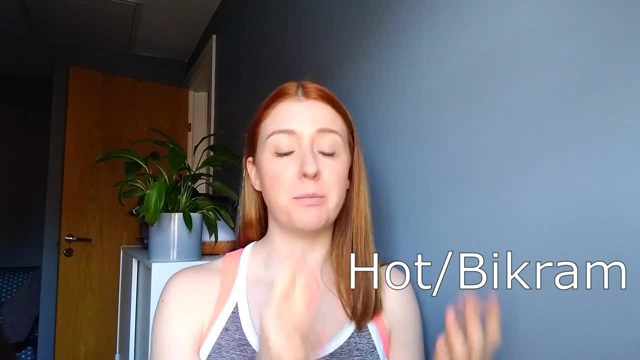 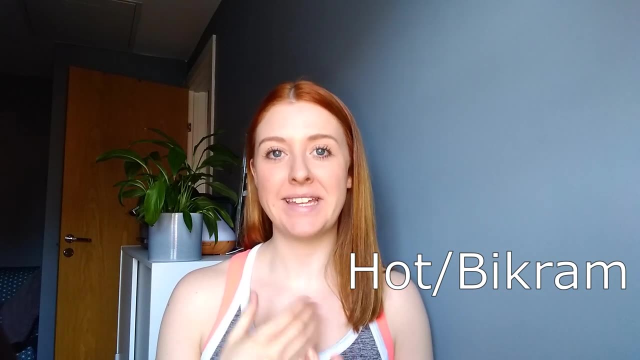 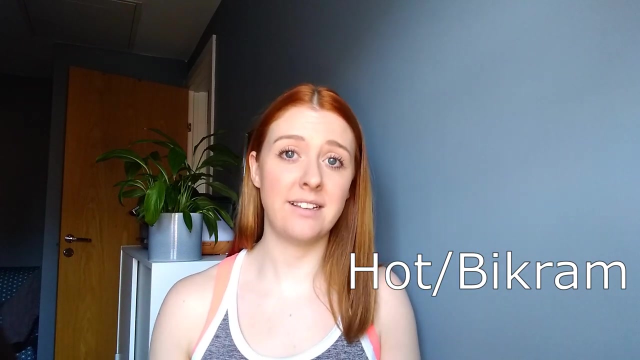 them together and it's hot yoga and Bikram yoga. Bikram, again, is named after the man who founded this style of yoga, but it has, within recent years, come to light that he is a very problematic man. He was very, very big in the yoga world, across the world actually. He still is alive and teaching. 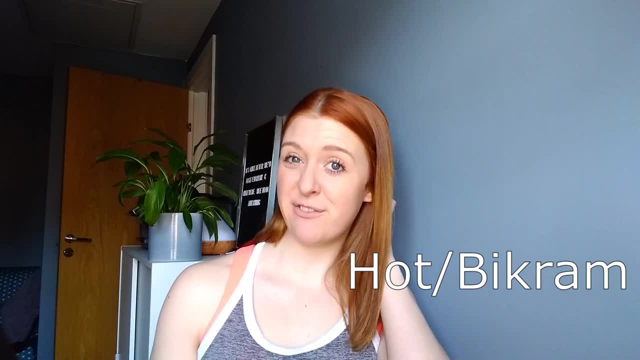 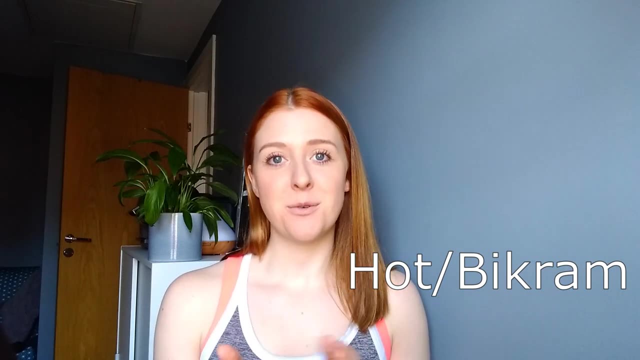 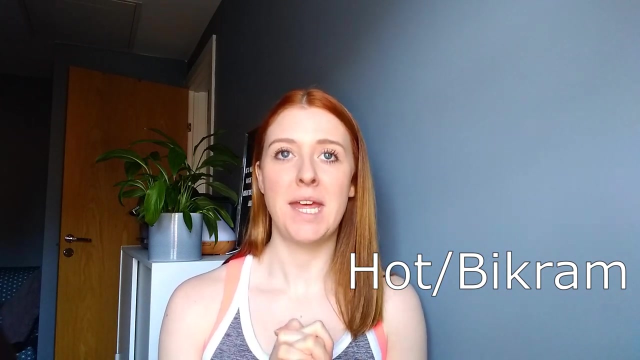 but as he rose to kind of fame within the yoga world, he abused his powers and was very abusive to people. So, as this has all come to light, if you want any more information about that, it's all online. There is even a documentary on Netflix at the moment about him. But if you have 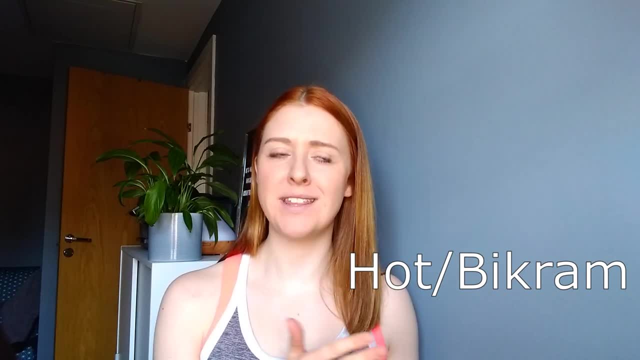 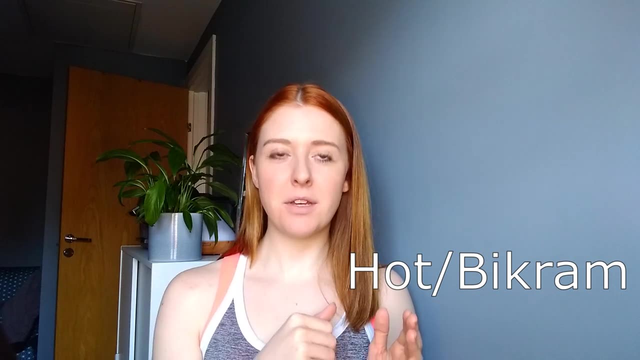 been to a studio where they offered Bikram yoga in the past and you're wondering why they've stopped offering Bikram yoga, then that might be the reason A lot of studios are now moving away from the name of Bikram yoga. Bikram yoga is very rigid, very structured format. You practice a 90-minute class. 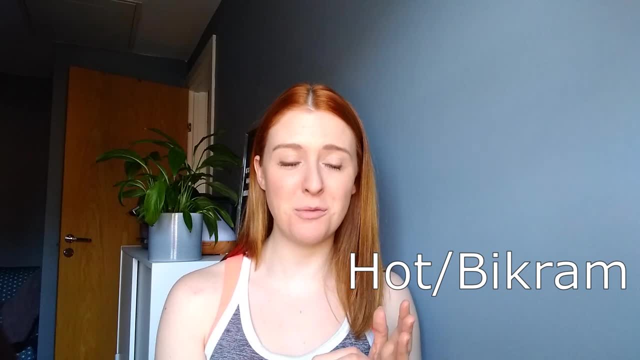 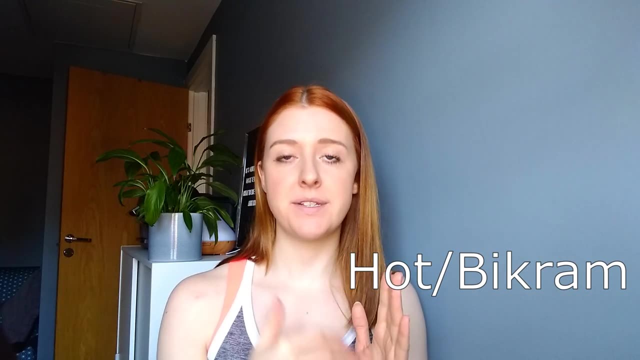 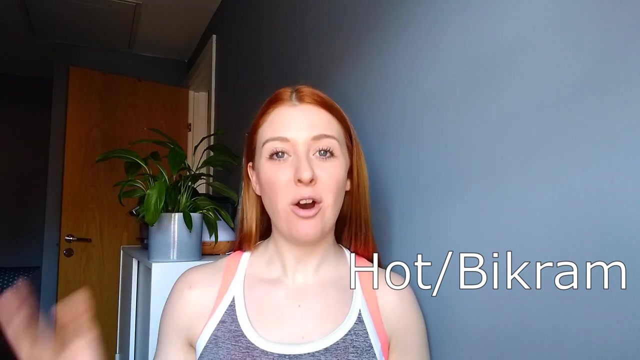 in a room heated to about 40 degrees Celsius. I think It's a very, very hot room. There are 26 set poses that you do and two breathing exercises, and that's it. So it's the same poses every single time in this very, very hot room. It's very, very intense, very physically and mentally challenging. 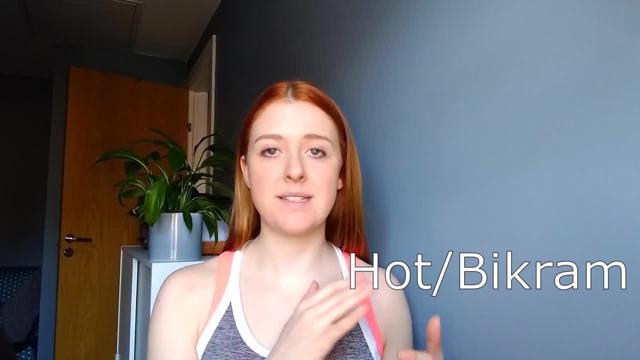 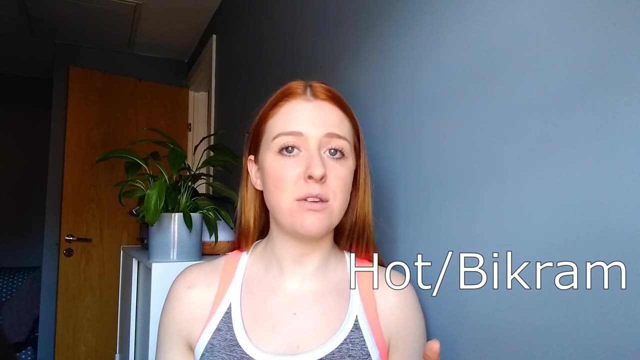 Then hot yoga. the only similarity really is that it's in a heated room. The rest of the structure of Bikram yoga is just Bikram. So in a hot yoga practice it depends where you go. it could be any teacher, any sequence of poses. It tends to be the more flowing style of yoga. 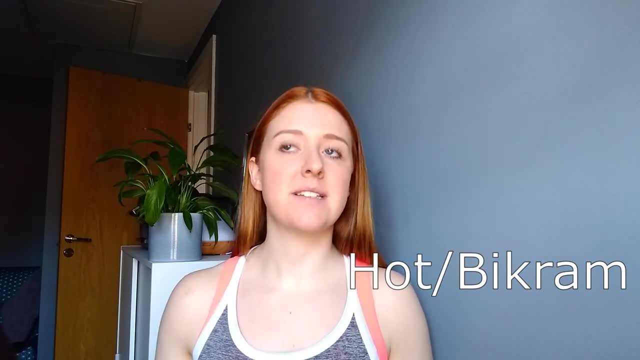 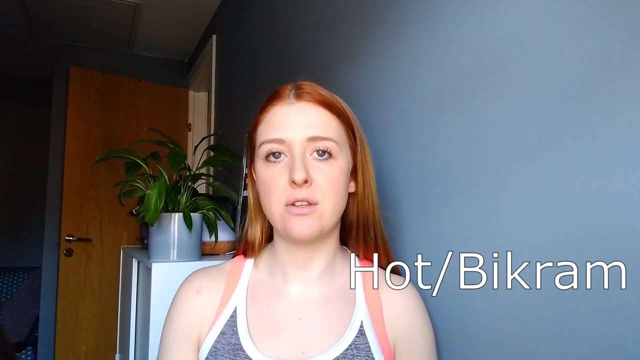 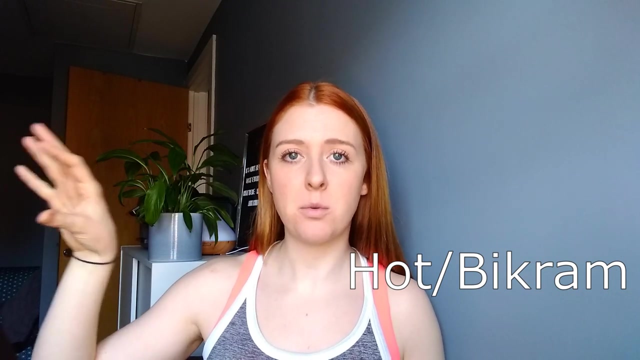 so a flow or vinyasa class, But it doesn't have to be 90 minutes and it doesn't have to be 40 degrees- It depends where you go- but the room will be heated to whatever temperature they advertise in their timetable And a lot of places now are offering hot yoga where it. 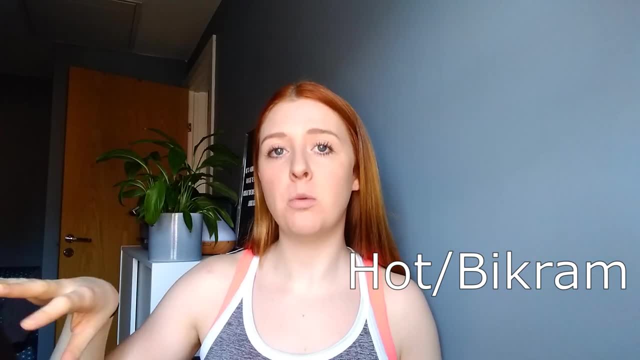 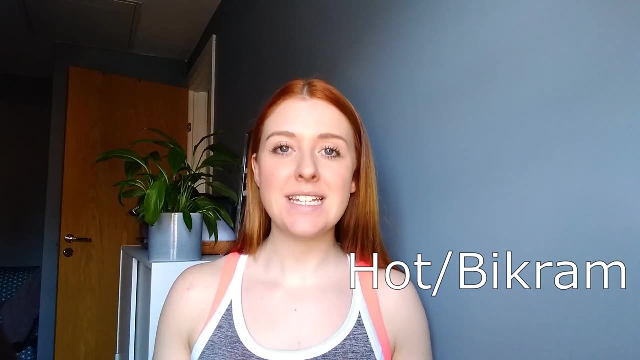 is quite hot, so say between 30 and 40 degrees, and then warm yoga as well, where it's more between 20 and 30. So that's a little bit more manageable for some people. So the idea of being in a heated 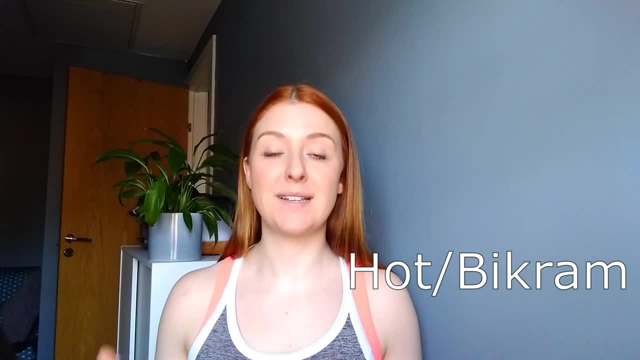 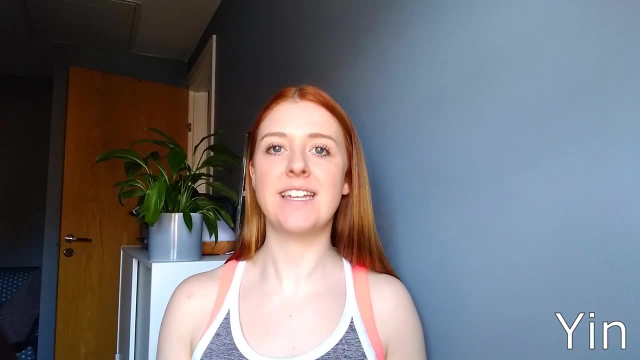 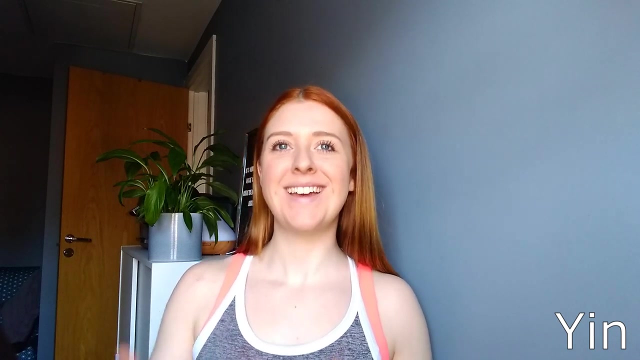 room is that it allows your body to open up more easily, for your flexibility to improve. And then, finally, yin yoga. So yin is quite different from all of the others in that it's a very slow, restorative, relaxing practice. With yin yoga you stay very low to the 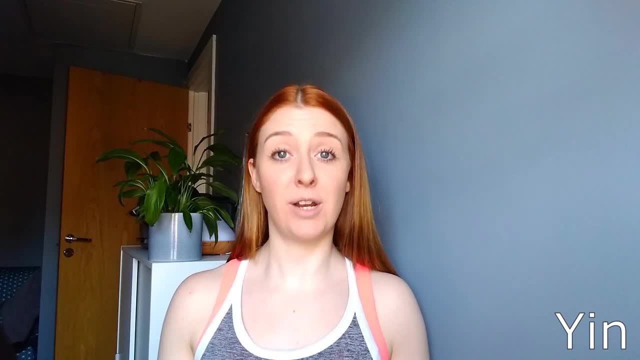 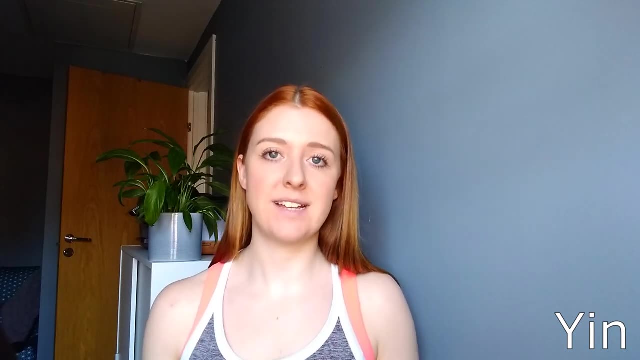 ground, because each pose you come into you're going to hold for a long time. So you'll come into a pose that doesn't require too much strength to hold. so it's more about the flexibility and about opening up rather than building strength. You're not going to be doing handstands and things. 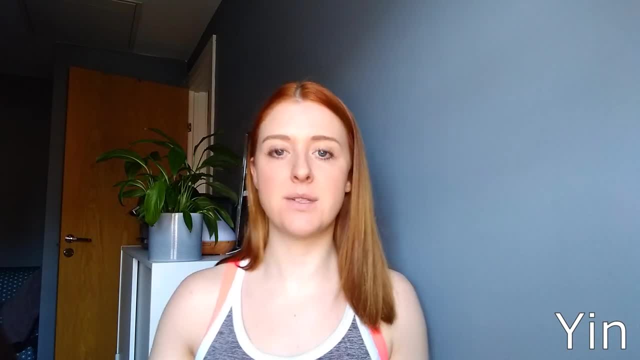 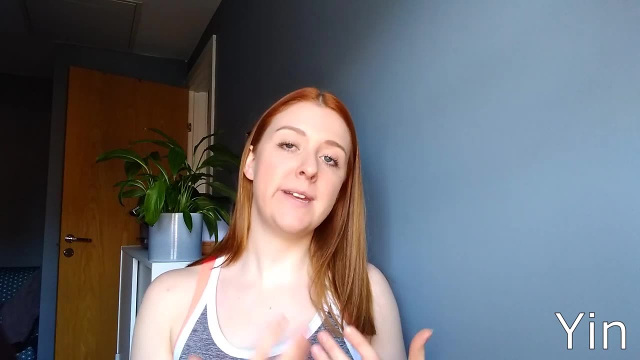 like that in a yin class. We use a lot of props and things in yin as well, so blocks, blankets, bolsters, big cushions so that you can get into position, And then the idea is that you will breathe deeply and you will relax into that.